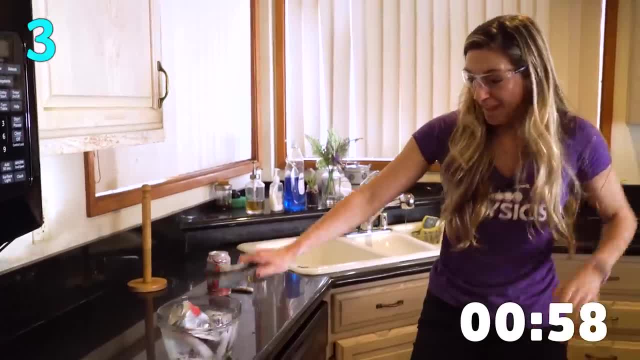 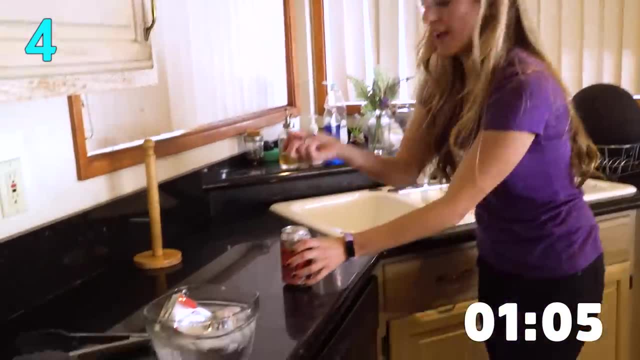 There's water in it. I'm going to turn it over into this ice water. Ah, and it crushes because of the pressure of all the atmosphere. Oh, I still need my safety goggles for the next one. This can is closed. I've got a Sharpie here and I'm going to just rub with some pressure along the edge over and over. 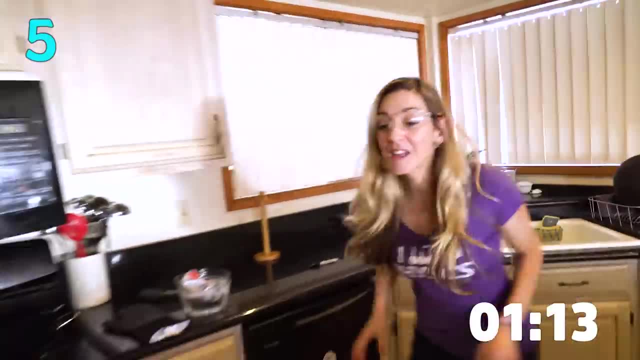 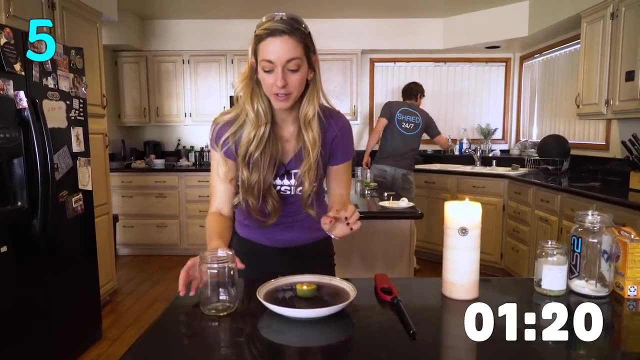 Oh, until it pops open, Love that one. Okay, the next thing: we've got the land of fire over here, So we've got an experiment with a candle, a bunch of water around it. I'm going to put this jar over that and we're going to wait a second to see what happens. 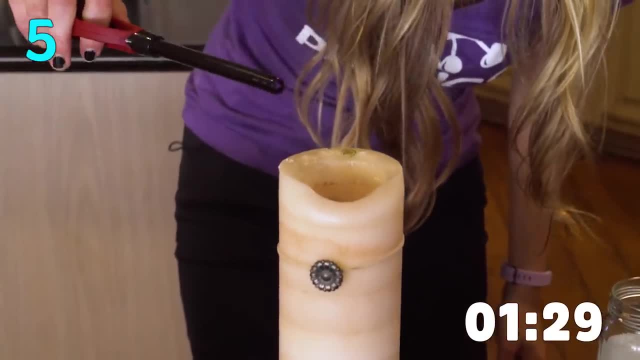 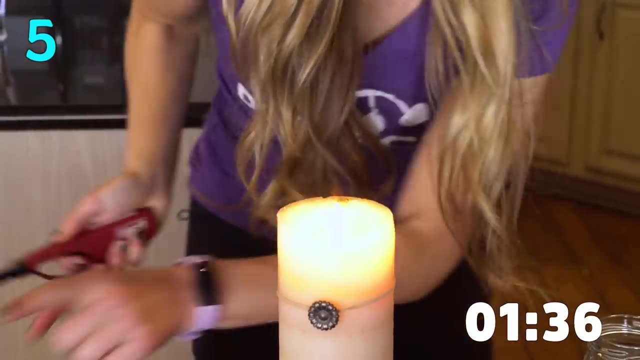 But first I'm going to blow out this candle and you can see that you can relight the flame. Oh no, I think I blew it too hard. I'm losing time. Check out this one in the meantime. This one's going out. 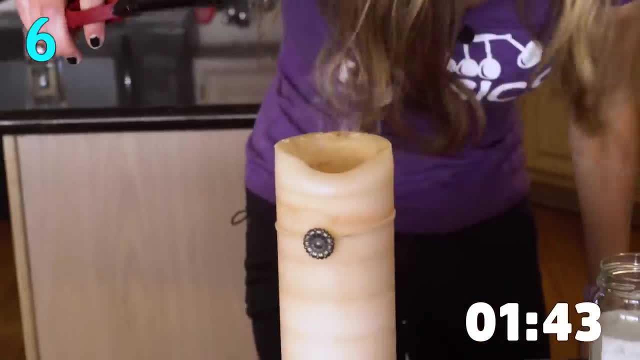 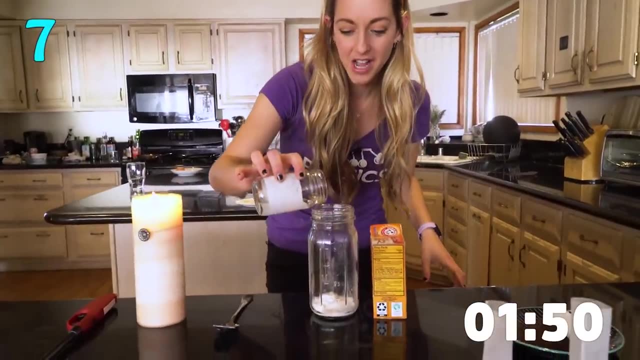 And the water level goes up because the air inside shrinks. Let's try this one again. Alright, you can relight the candle, Yes, But I'm going to put it back out With baking soda and vinegar. I'm not going to pour the vinegar on it. 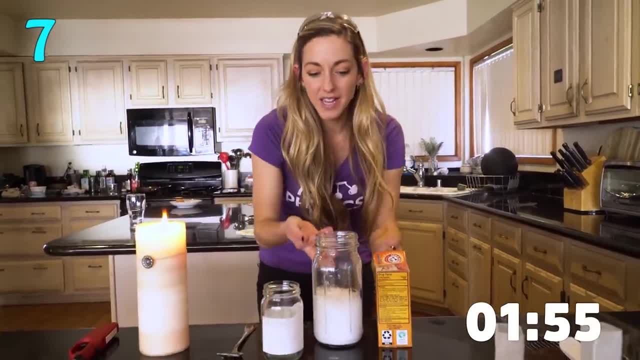 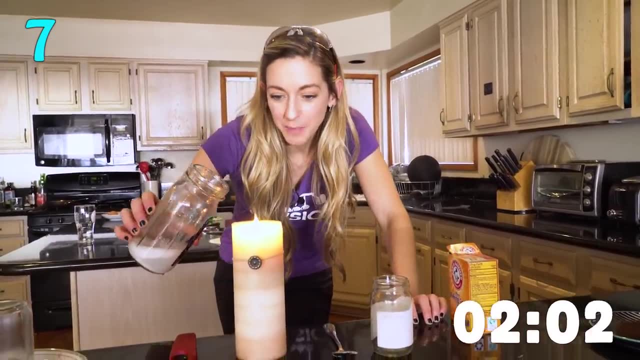 But we've all done this experiment. You create a bunch of carbon dioxide bubbles when you combine baking soda and vinegar, And carbon dioxide has the benefit that it is not oxygen, So you can pour out fire. Did you see that? It didn't even look like I did anything. 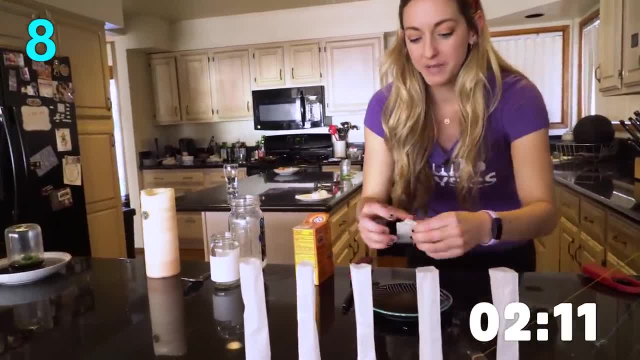 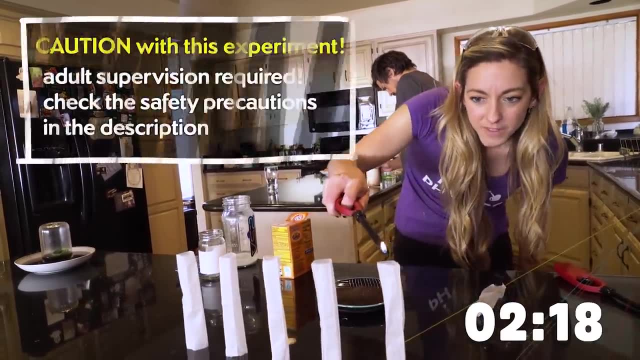 And the flame went out. I am losing time. Okay, the next one. If you take a tea bag, like cheap Lipton tea, whatever, Dump it out, You can make these little cylinders, Light them on fire And then, as they heat, up, 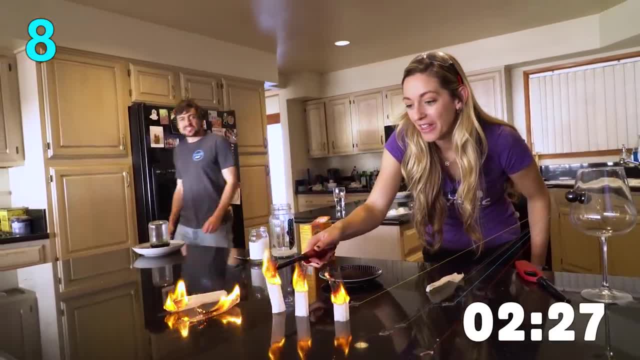 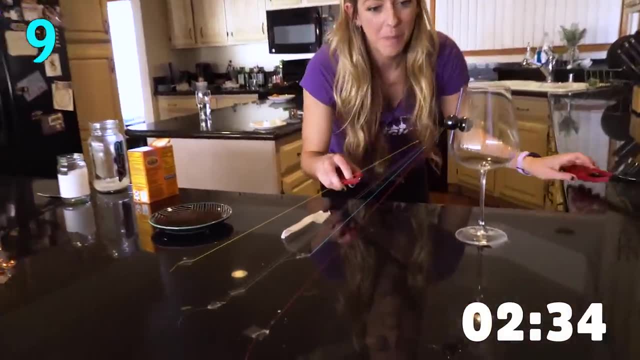 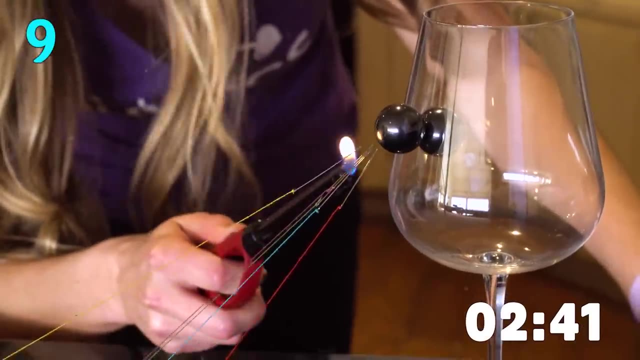 Oh no, As they heat up, they get lighter and lighter And then they start to fly, because hot air loves to rise. I've got a bunch of needles pointing at this magnet And they're all attached to strings. I'm going to heat these up. 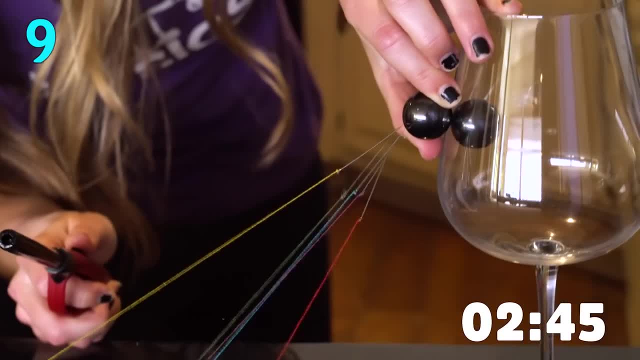 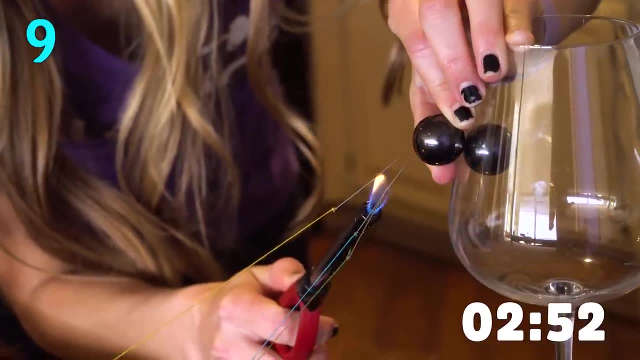 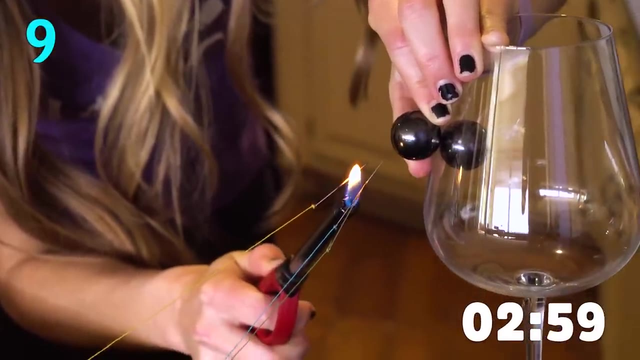 Oh, shoot, No, No, Okay. Oh, we're still good. We're still good, We've got a couple. I'm going to heat these needles up And, as I do, They're going to lose their magnetism. 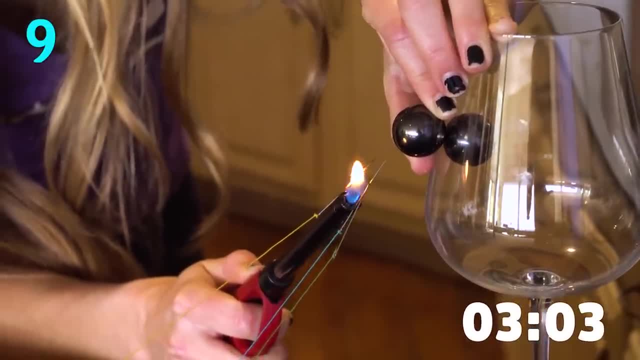 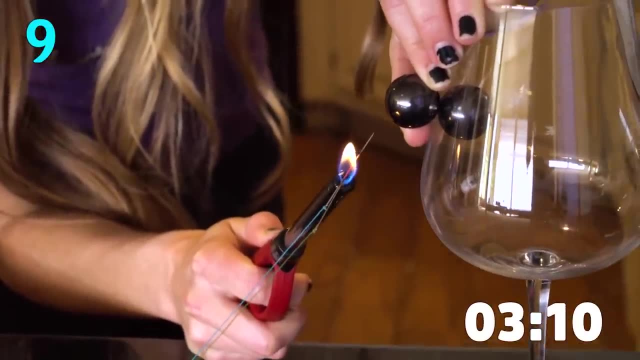 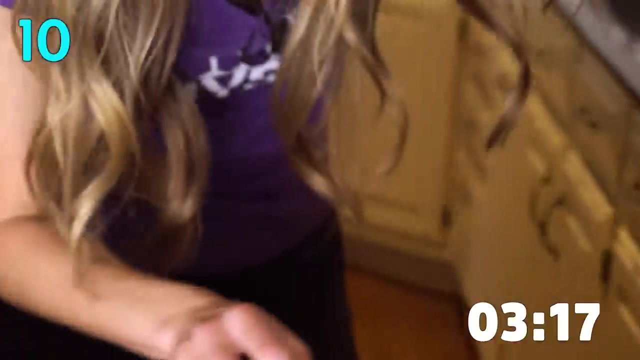 Because they get above Two minutes, Oh my God, Where metal stays magnetizable. And they Getting close on that. That's really cool. They, Oh my God, They fall, Yes, Yes, Okay, Next one. 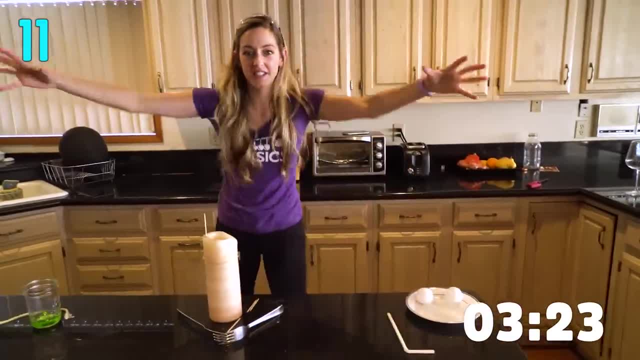 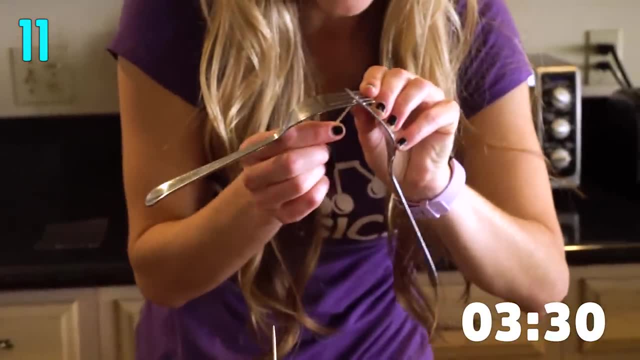 You can balance a ping pong ball on a stream of air. This is the challenge island. Right here We've got some interlocked forks. I'm going to take a toothpick and stick that through And use the principle of center of gravity. 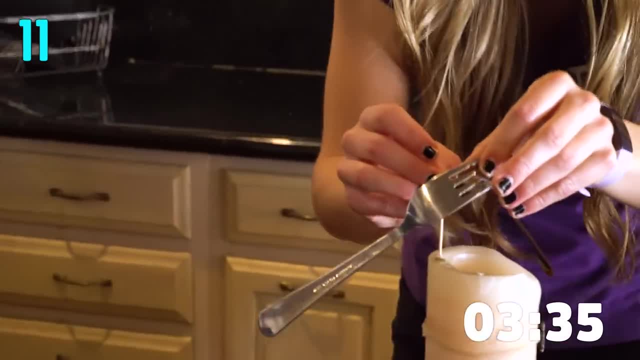 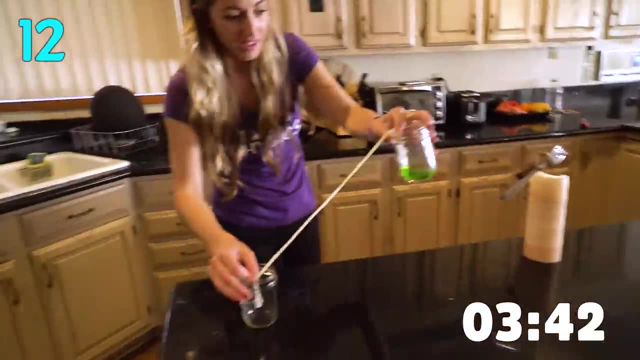 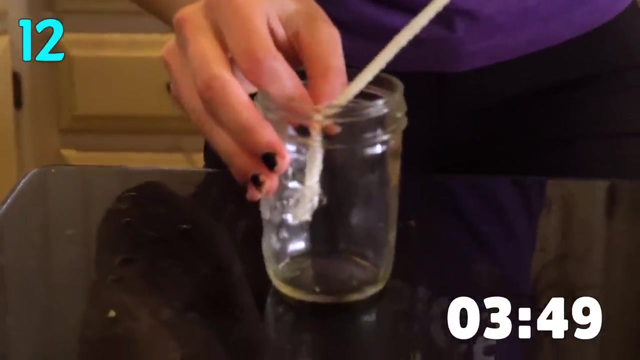 And get the center of gravity below These balancing points And I can Balance the forks- Amazing. The next challenge: I'm going to take this regular string And pour some water with food coloring in it from this cup, Using the properties of surface tension. 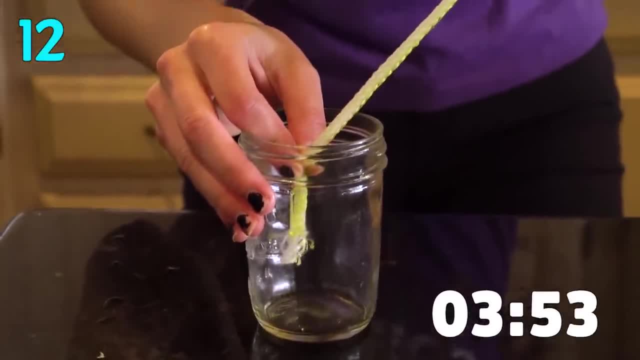 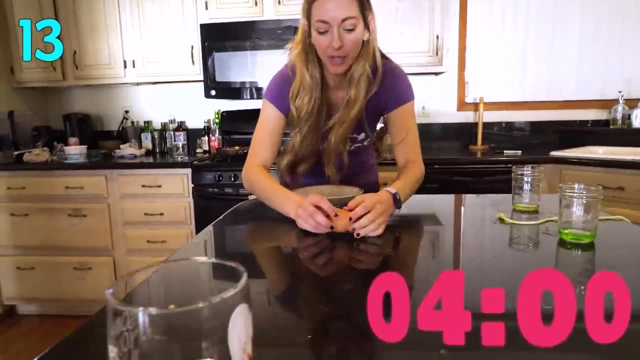 Down the string All the way to the other cup. I don't have time to do the entire cup, though You get the point. It's super cool If I take a hard boiled egg, Not a soft boiled egg. Oh my God, One minute And I spin it fast enough. 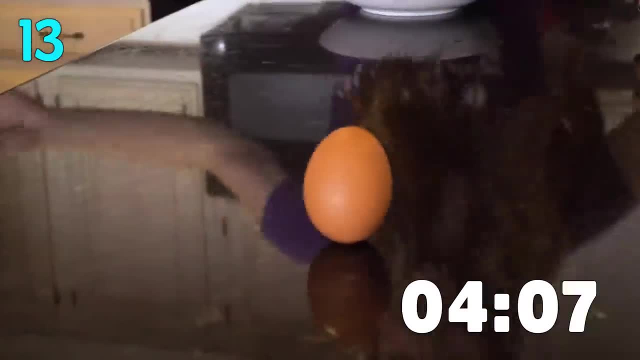 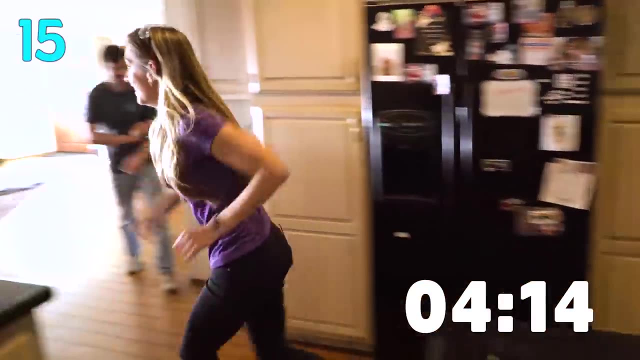 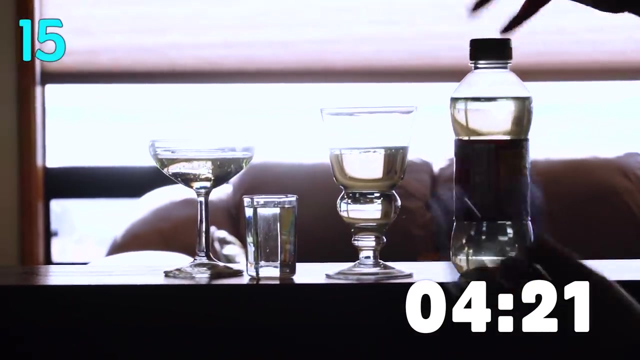 I can get it to stand up On its end. Amazing. Now take a card with a cup, Turn it over. It can hold up the cup. Excellent Polarizing sheets. You can look through them and see the properties of corn syrup. 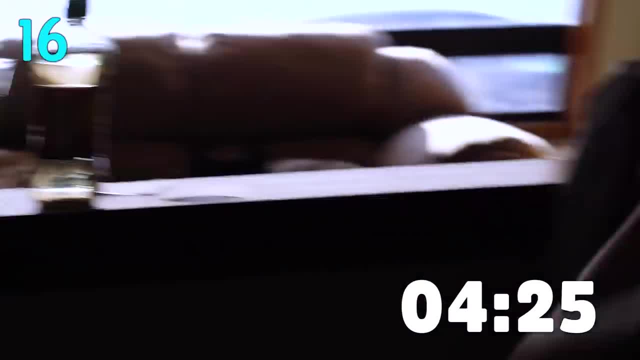 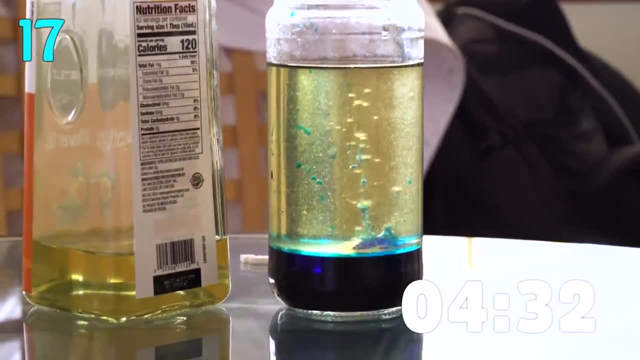 And how they've got amazing optical properties. Take an Alka-Seltzer tablet, Put it into some water With some oil on top And you can make your home lava lamp. Watch that I'm going to take this egg And show you the property of impulse. 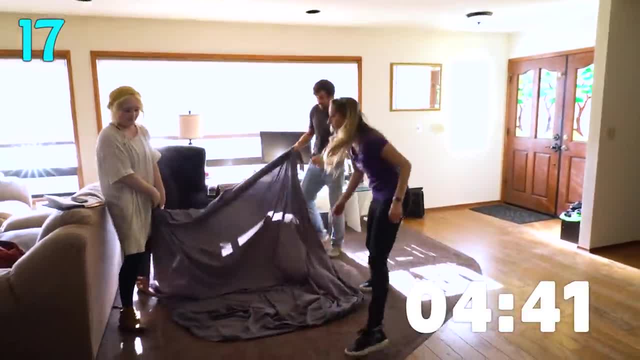 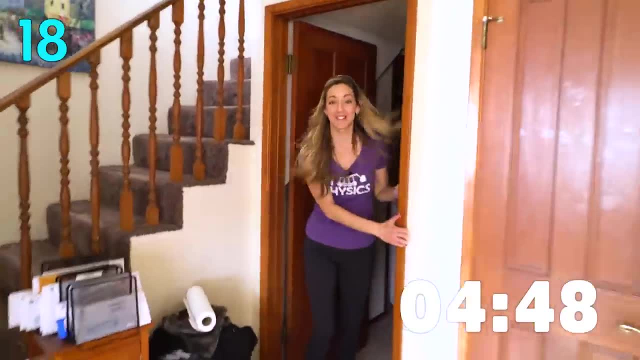 Which is that if I throw an egg, It'll get caught by something with give, But if I throw it with something with not give, Someone's going to have to clean that. And here I've got a non-Newtonian fluid. This acts like a solid. 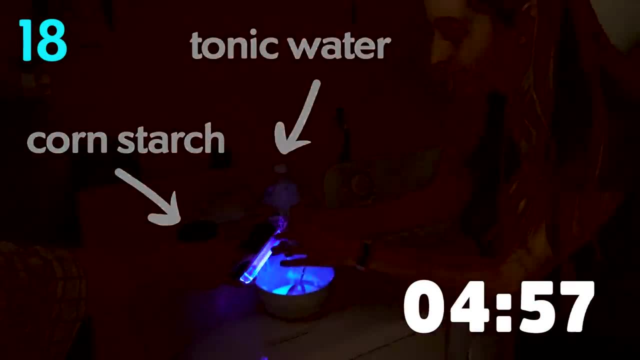 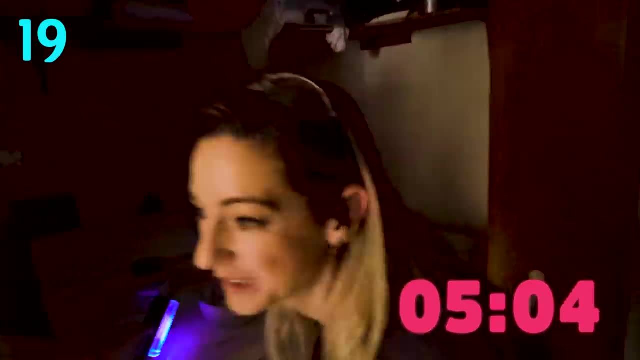 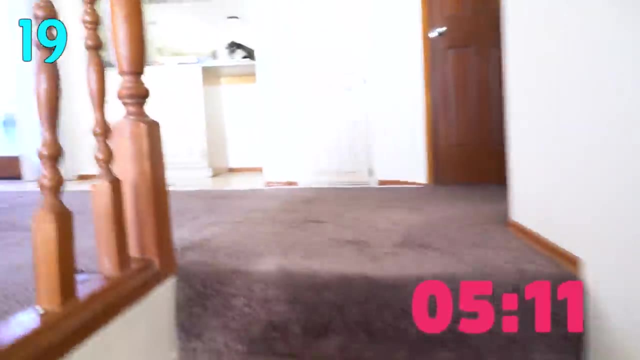 But then it'll act like a liquid As soon as I let it flow. What are we at? Five minutes, No One experiment. We have one experiment left, Okay. This one uses the principle of inertia. We've got these eggs here.